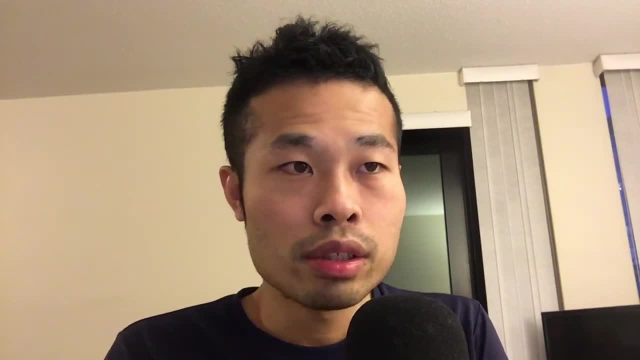 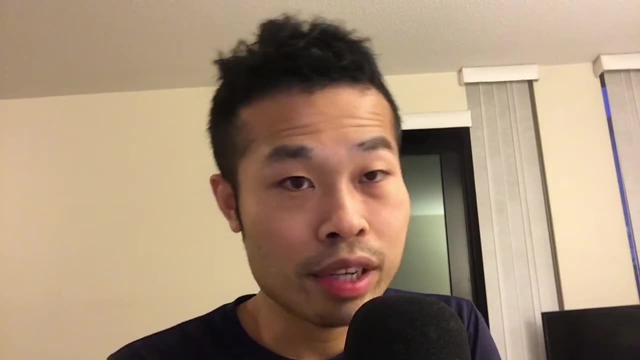 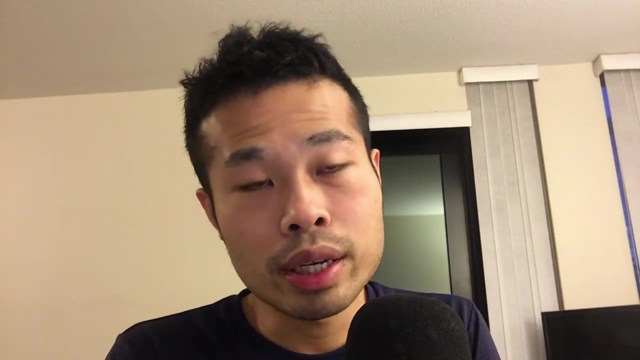 so many things that you can do with computer vision. So the majority, like I will say, is probably after. like over 70% of AI job markets are about this category: computer vision, And another category. it's also popular, but much. 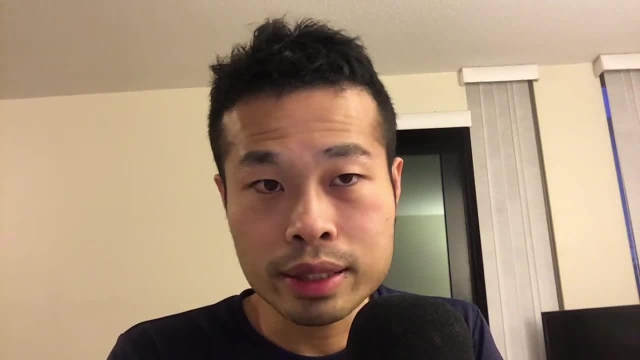 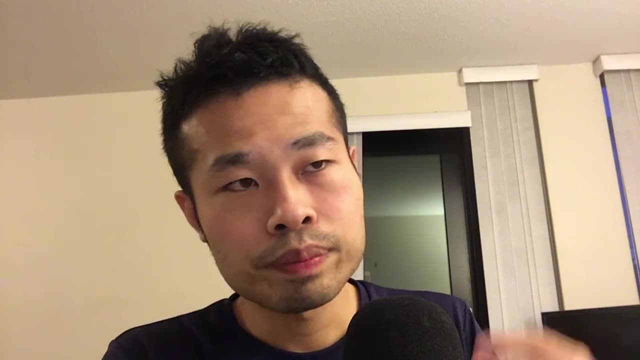 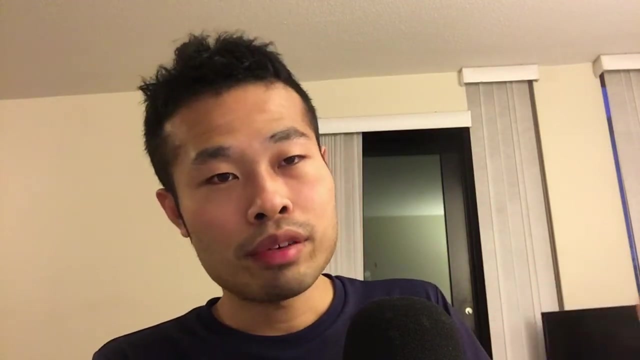 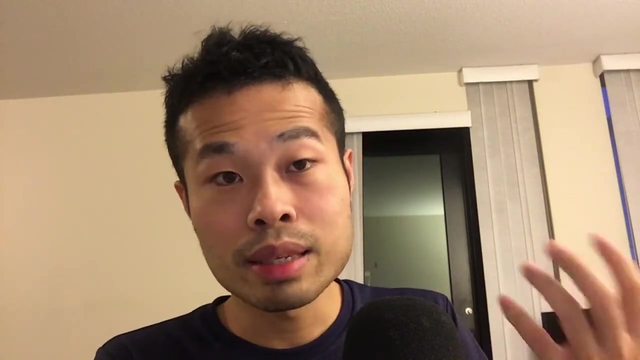 less popular. It's natural language processing. Natural language processing is basically the domain that people process Human languages, for example English. if I'm saying something now, the natural language processing will analyze what I say and to maybe analyze my emotion, my sentiment or my intent of this speech. 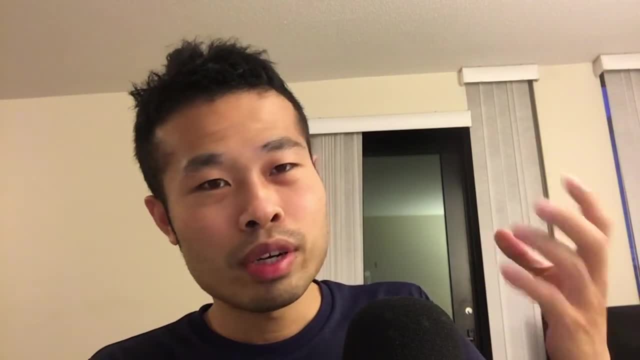 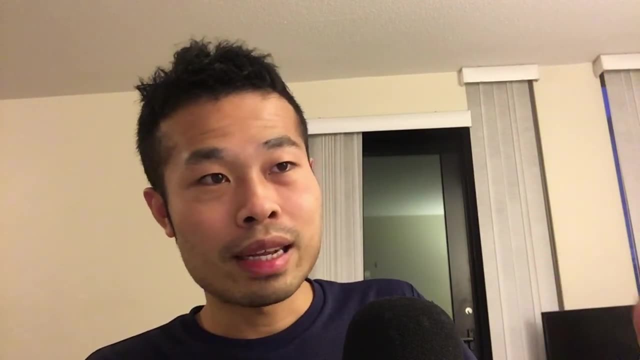 that kind of things, And you can apply that to spoken languages, you can apply that to written languages, So that's, like I would say, the second most popular one. but it's like, far from computer vision, You can also see these phenomena from the. 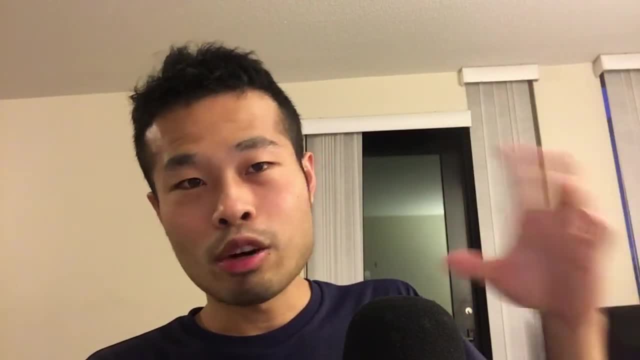 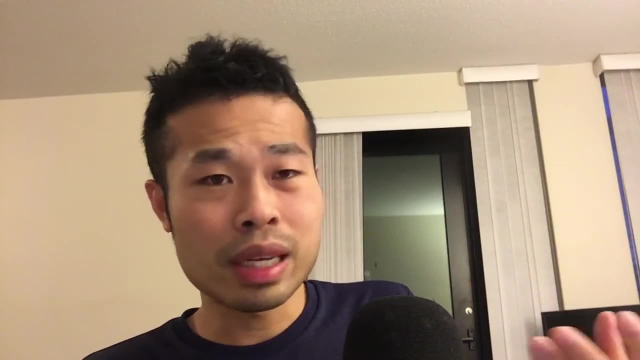 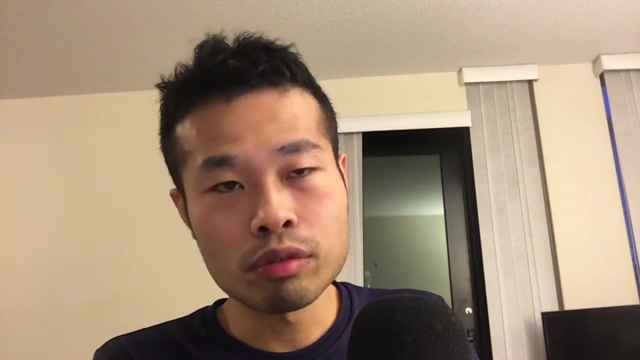 papers that are published every year, Really really over 60, 70% of papers are about computer vision And as far as NLP, it's probably like 10 to 15%. Okay, another domain is also popular is robotics. Robotics is where you use you use AI to 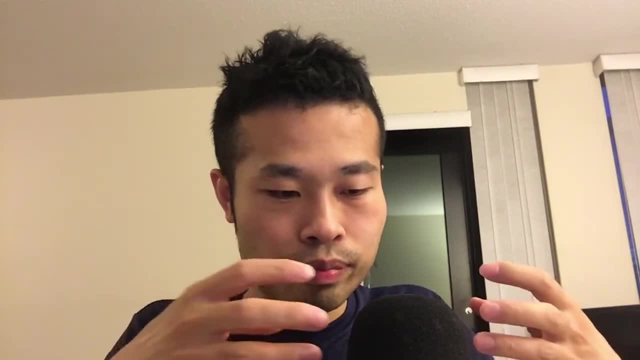 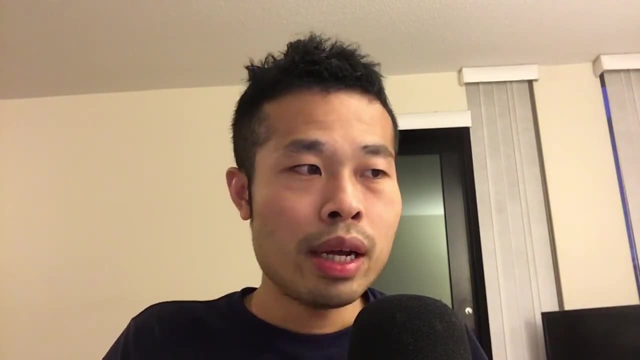 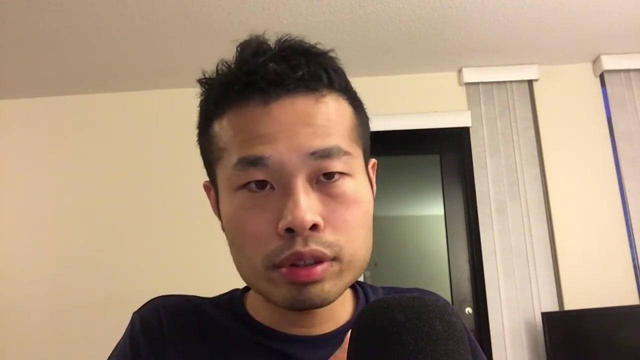 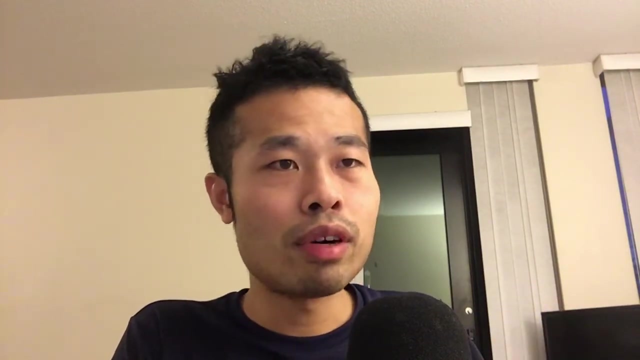 control or to- yeah, basically to operate the robots. It's robotics or like a robotic arms. they can control and it requires a lot of reinforcement learning, And this branch is also also like something and people use these to do. you can say self driving cars, one of these relative things, or 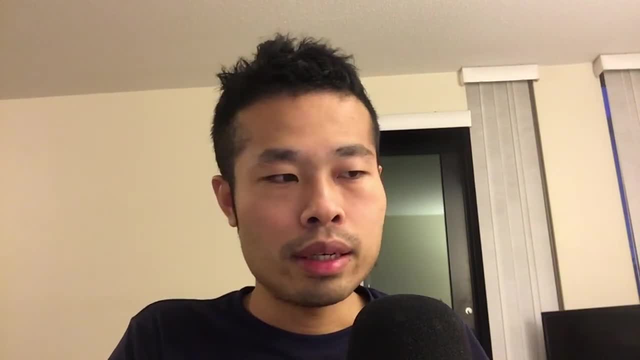 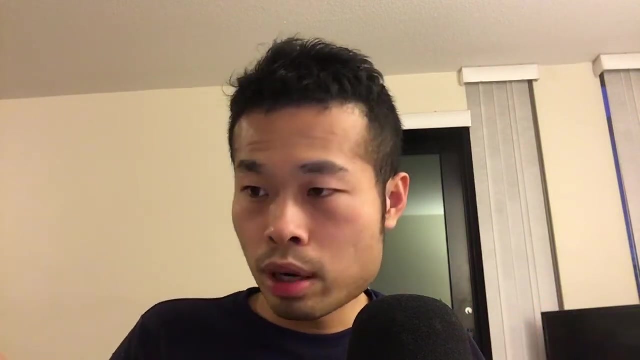 like industrial robots, They kind of things. Okay, so these is robots and other another one I would say speech recognition, auto automatic speech recognition. it's also popular. for example, if you're watching my video now, you will probably see there's a CC button on YouTube. if you click that, they 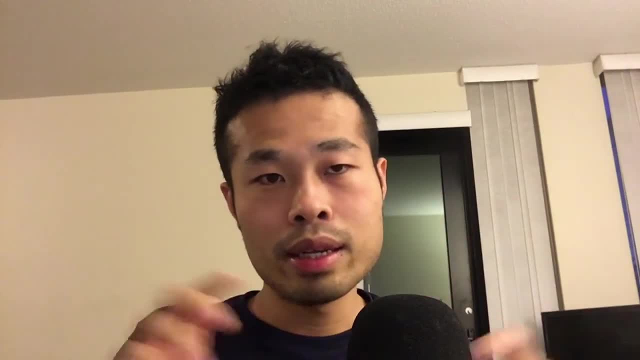 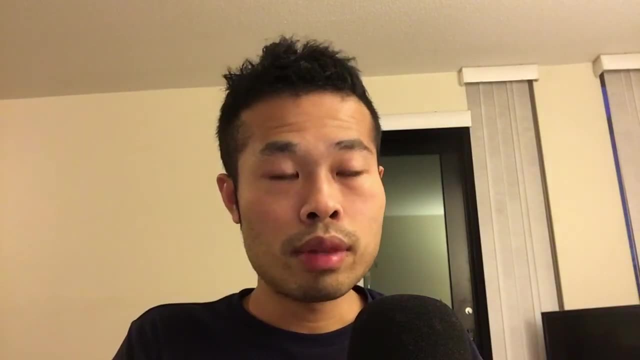 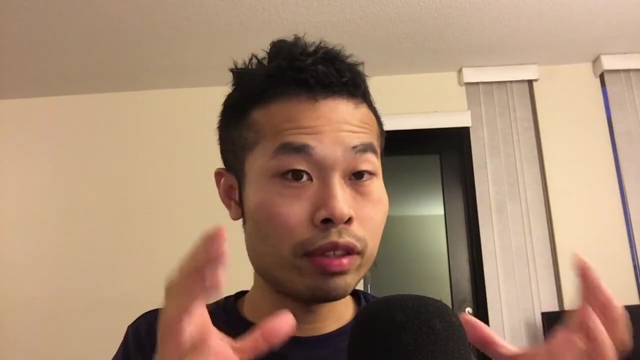 would have. they will show you the transcript, which is done by an ASR model. there's just a transcribed by a machine learning model. so this can have a lot of applications as well, because if you want to use NLP to analyze spoken languages, you first of first of all you need to transcribe it. 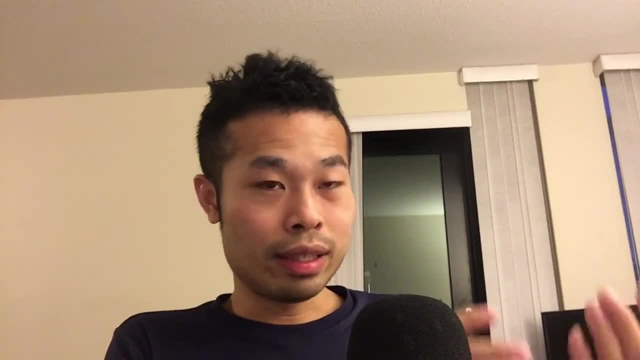 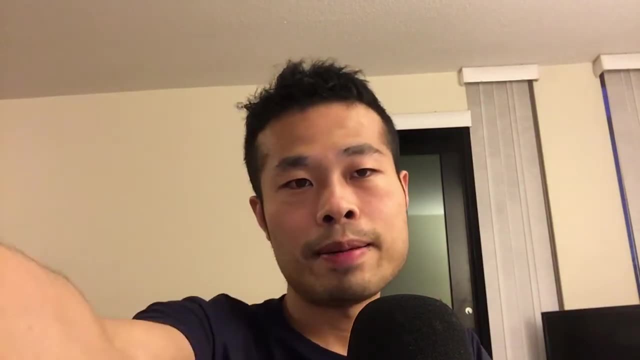 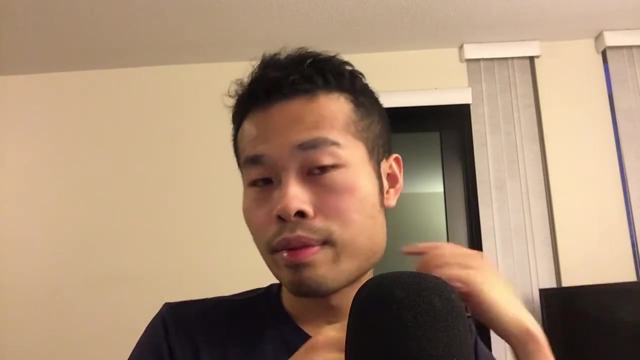 then you can use NLP technique- natural language processing technique- to process a transcript. the transcript okay. so that's ASR, and there are ASR also improve a lot, like during machine learning big revolution. you can use NLP to analyze spoken languages and then you can use NLP to 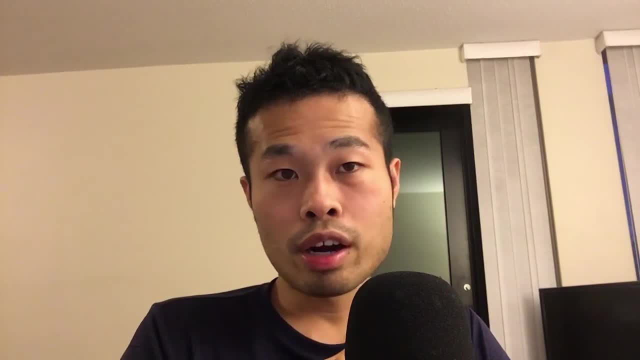 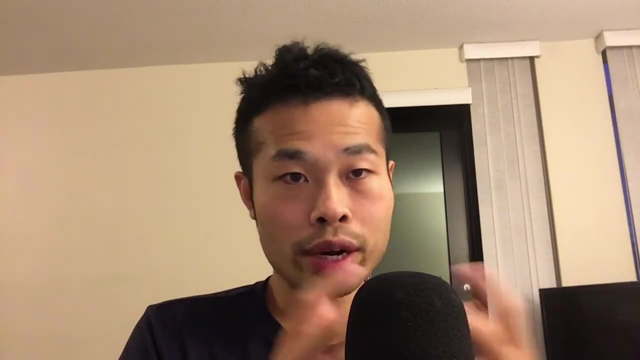 analyze spoken languages. so now, if you look at the state-of-the-art English is ASR model, speech recognition model. it's almost as good as humans, or even better than humans- I would say what? but still, this domain, there's still a lot of things haven't done yet. for example, foreign accent like I'm. I'm saying I'm. 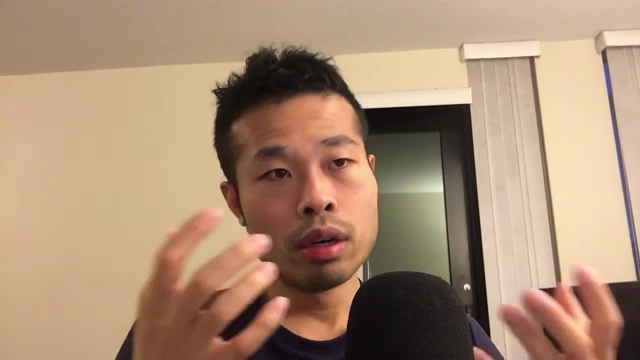 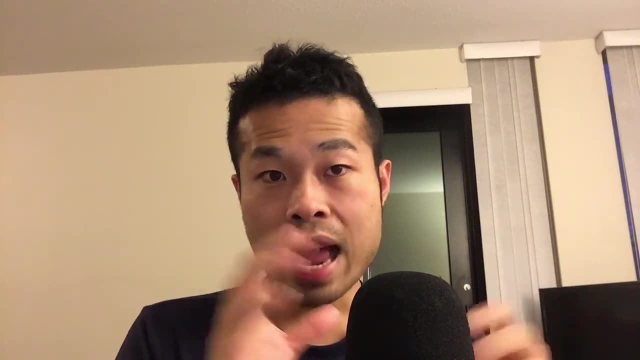 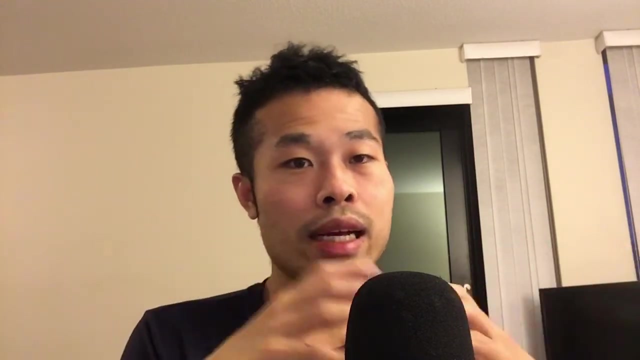 speaking English. English is not my first language, so some ASR model if there's not good enough. they wouldn't be like transcribed my speech accurately. and also there are many, many different languages, so there's English is like high resource languages, so it's easily easier to do it better. 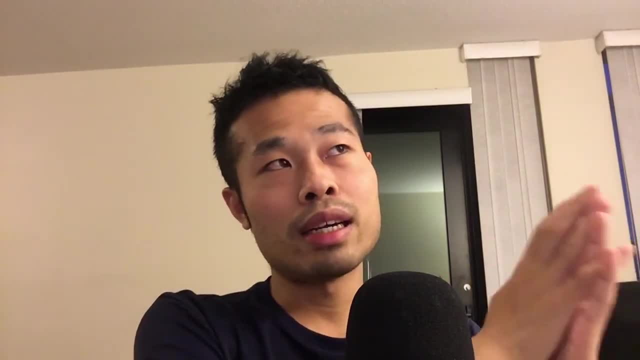 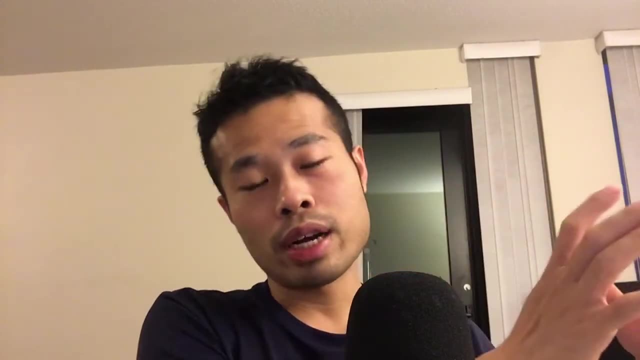 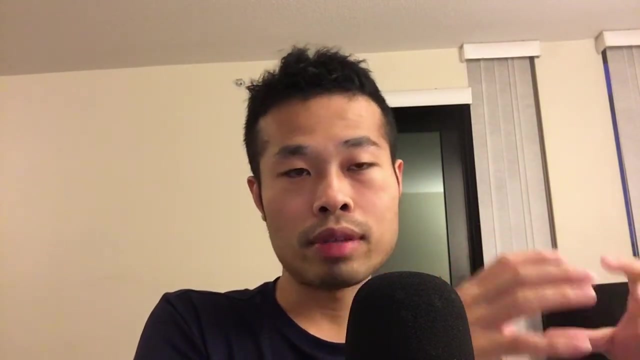 than the other languages. but if you are saying a lot of like other languages even, it's still a major language, but it's not English. once you go away from English, the resources much less. so. the ASR speech recognition accuracy is still not good enough, so there's still a lot of things to work on. so this domain is also popular, so 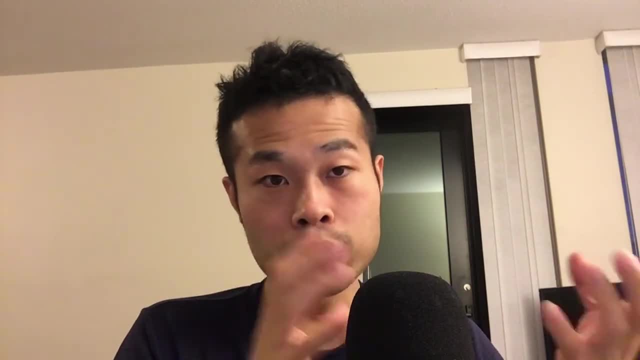 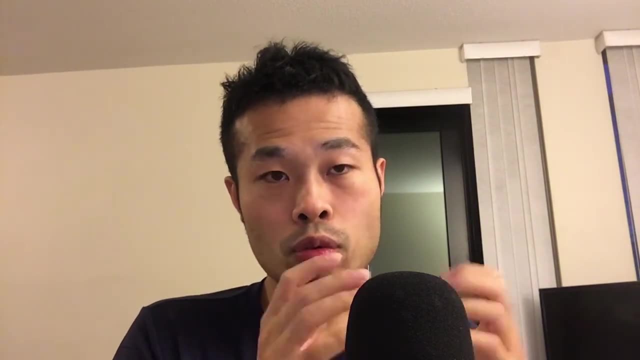 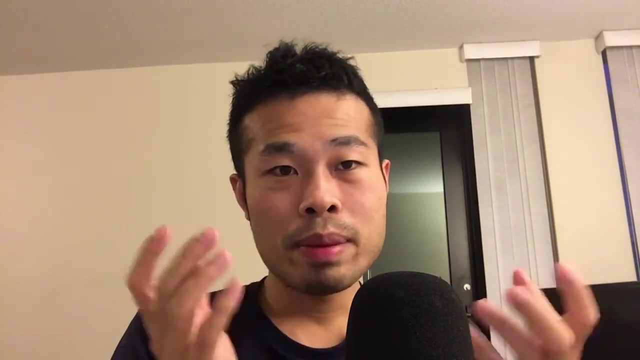 these are a few popular domains in AI, and I just talk about it by domain. and as for how you can go about it, if you want to work on, let's say, computer vision domain, NLP domain, ASR, robotics, they kind of things, maybe I will make a. 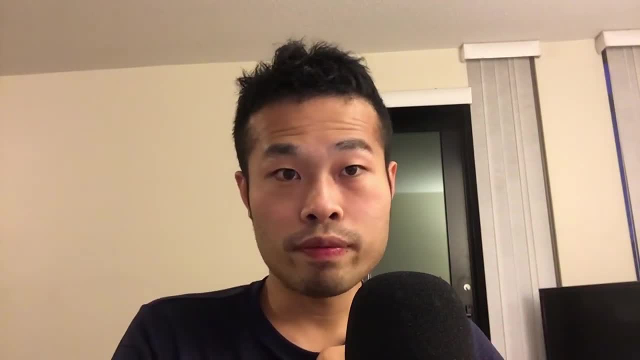 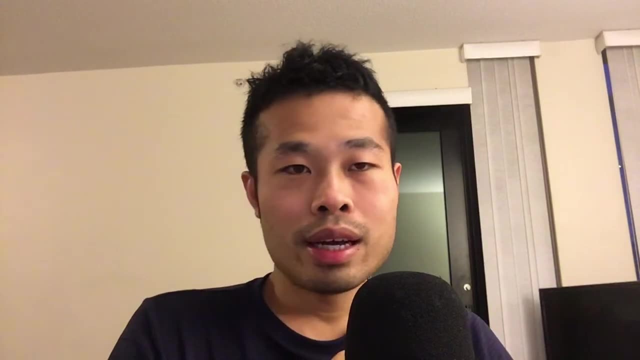 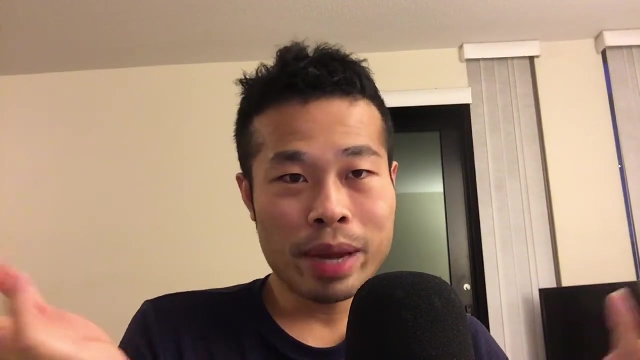 several videos to talk about it and I'm not really sure if anyone's interesting in this kind of video. so I just make this to test the water and see if it really got a lot of feedback or anything. then I could make more. I'm more than happy to make it more and have a like a lot of experience in.